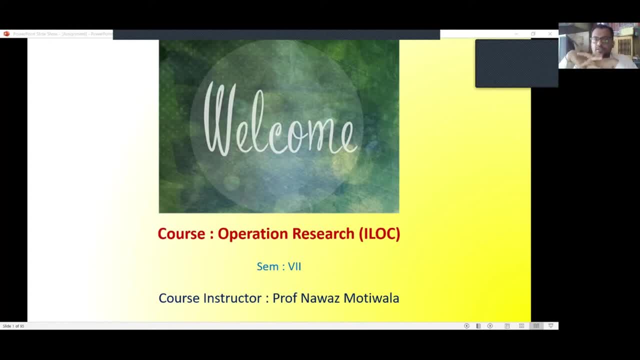 Good morning and welcome to all for this course on operation research. So before starting, can someone volunteer and tell me whether my screen is perfectly visible and I am perfectly audible? Yes, sir, Thank you. Okay. so normally there is a practice that in first lecture we introduce you to the course, that is, what is its application, what are its advantages, disadvantages, where the subject will be. 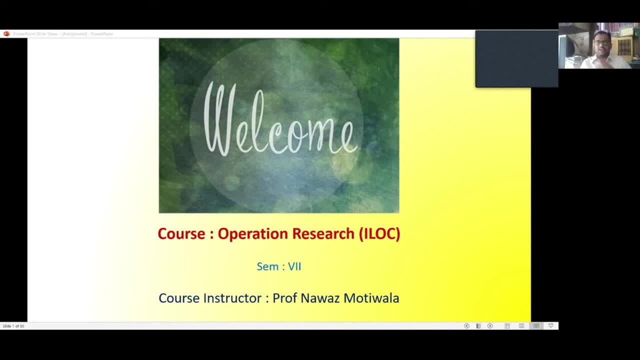 helpful to you in your career, etc. But this time I have tried something else, just by showing you PPT and making you bored in the very first lecture. So I have think something different, that I have compiled all that half an hour data, which would have taken if I have shown two slides. I have compiled it in a very interesting 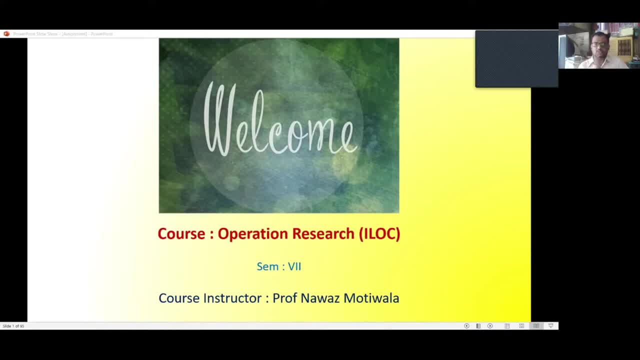 three to 3.5 minutes video. So now I will be playing one video in which you will be getting the entire glimpse of the subject, that is, what are its advantages, what are its disadvantages, applications, etc. And the interesting part is you have to be careful while watching that video. 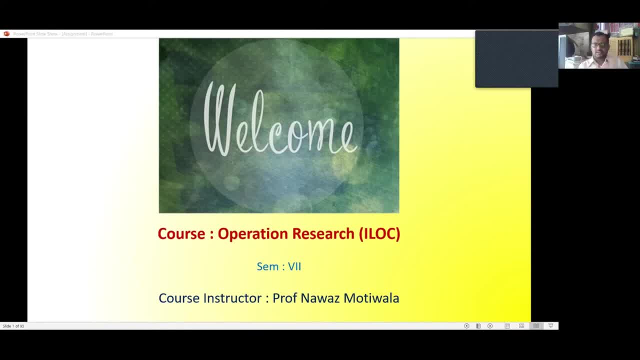 Because at the end of that video I will be posting one quiz on it which will be related After going through that video. you can easily answer that And, believe me, it will be an interesting one And you will enjoy the course. So are you ready for that? 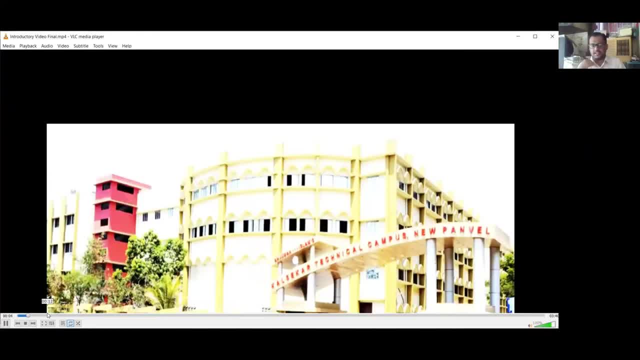 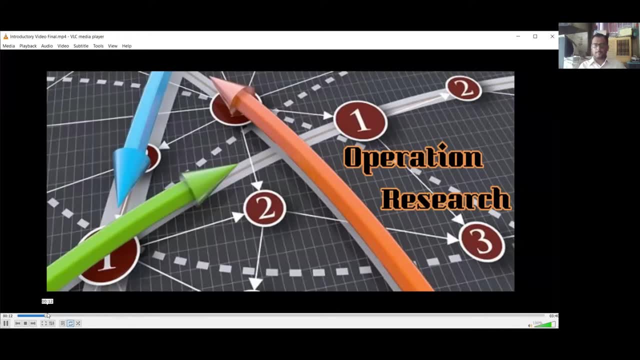 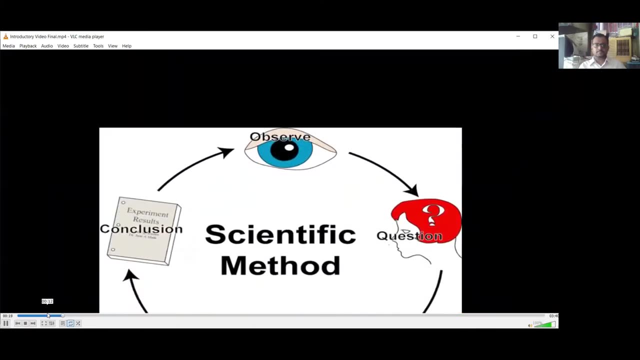 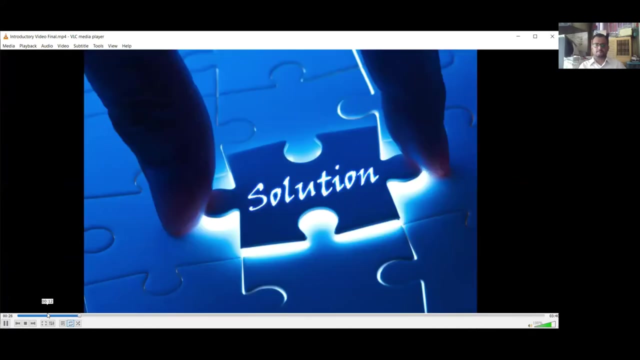 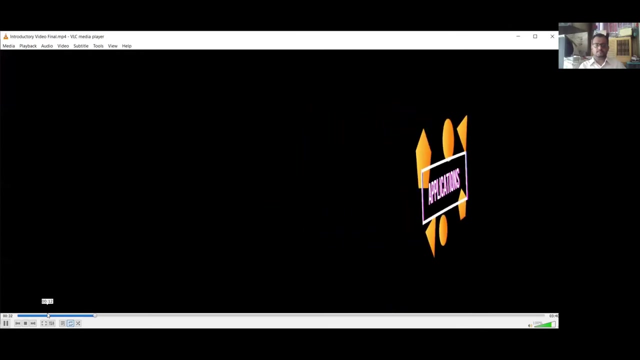 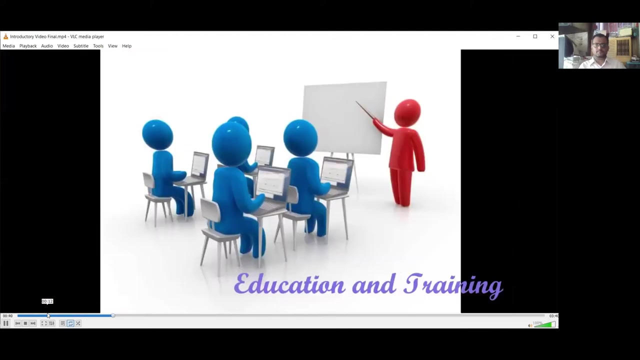 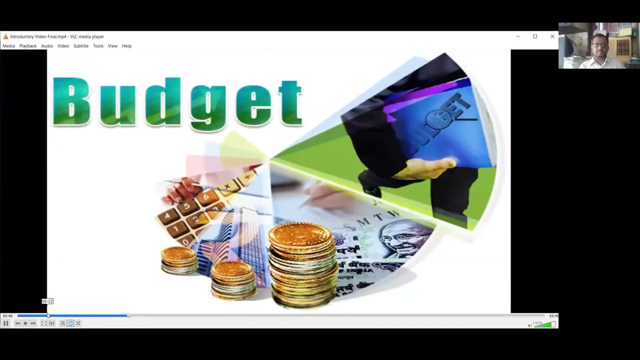 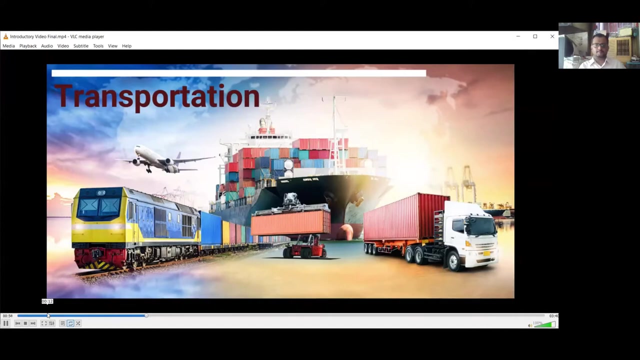 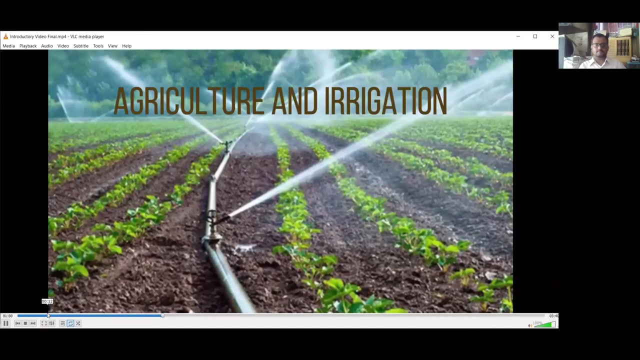 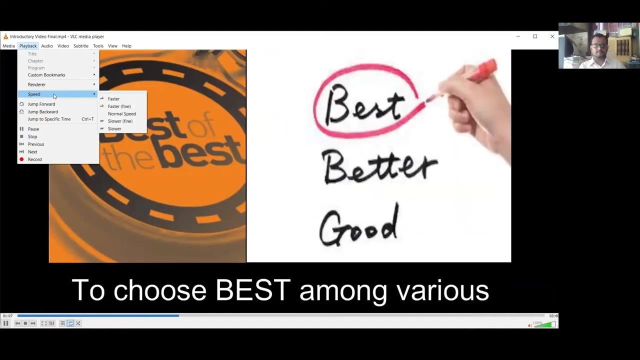 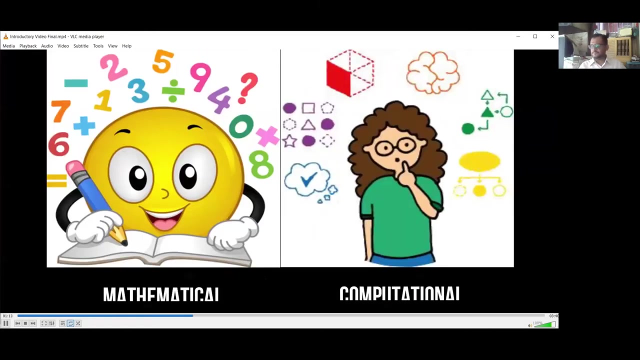 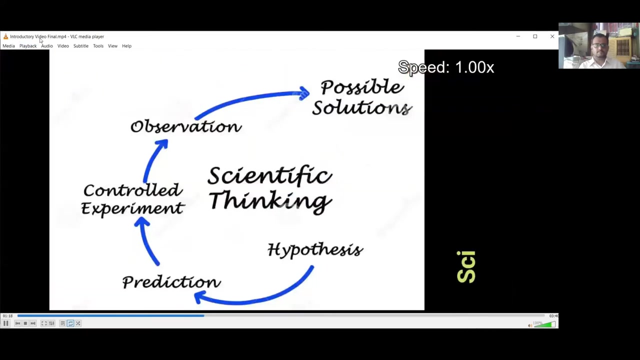 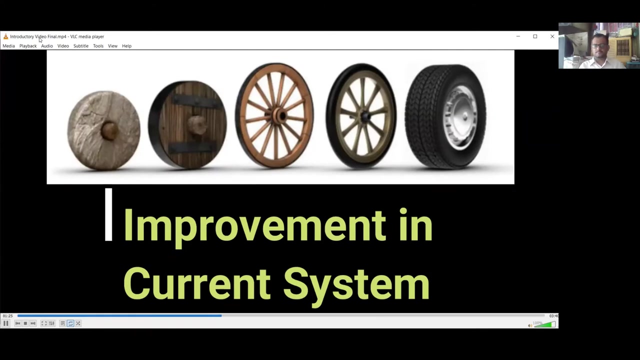 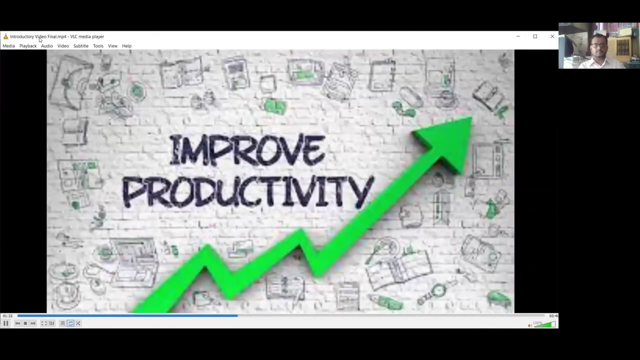 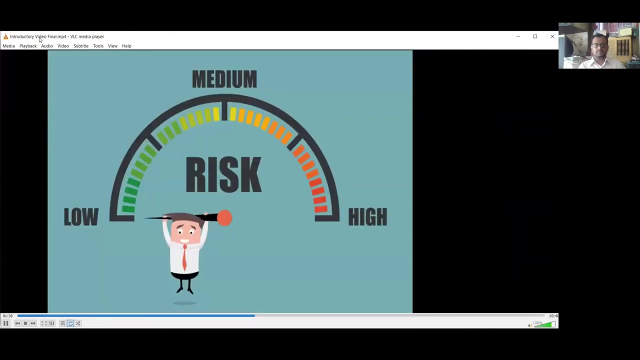 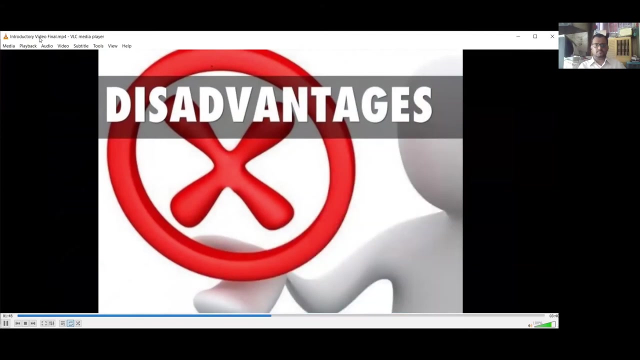 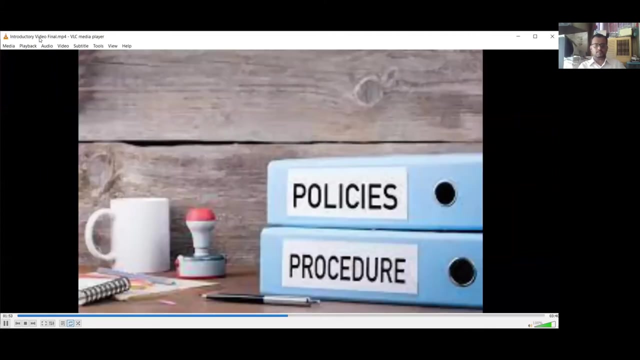 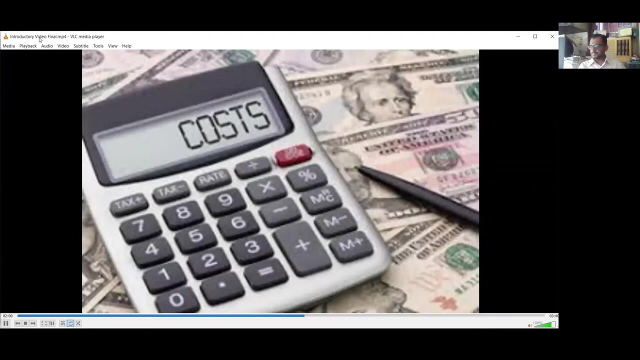 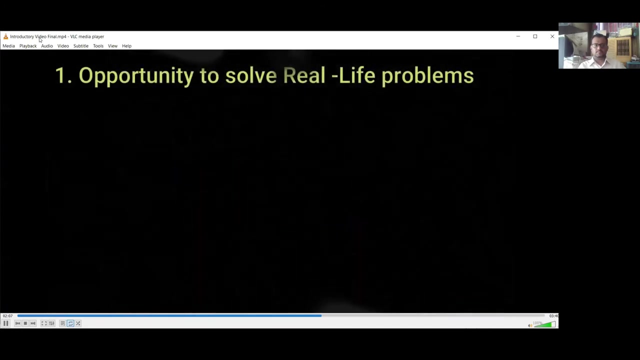 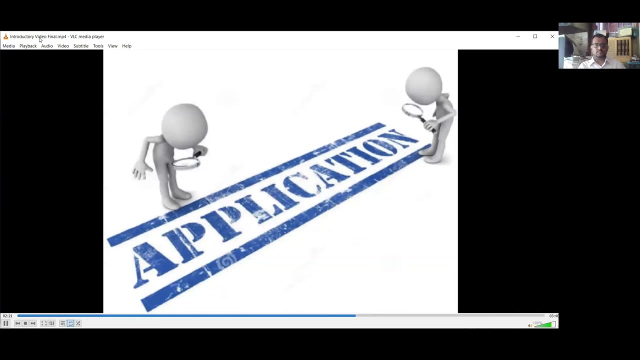 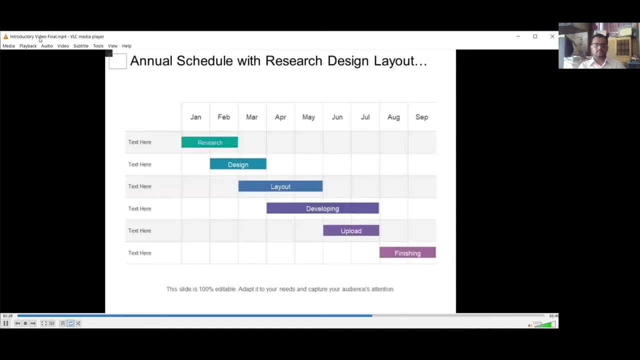 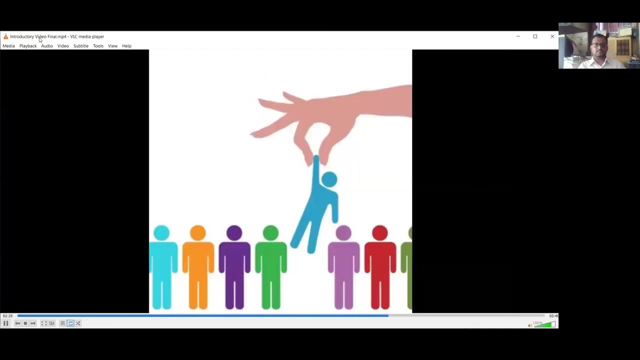 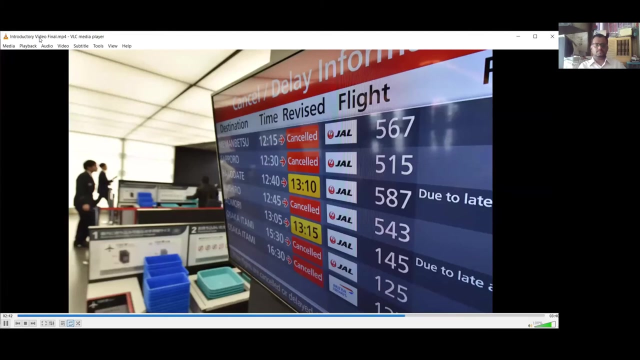 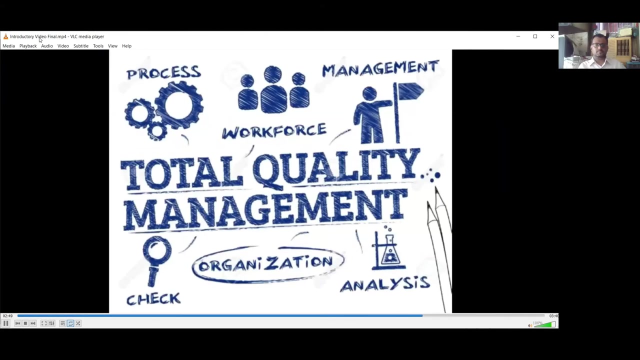 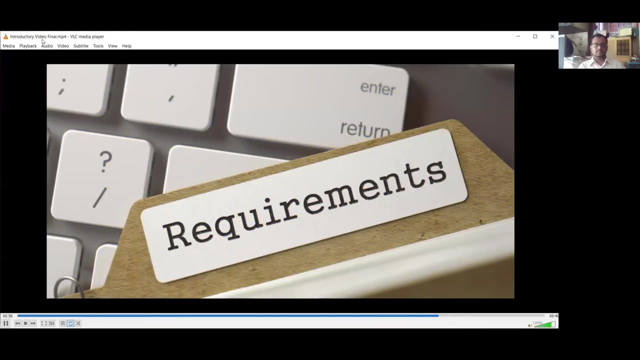 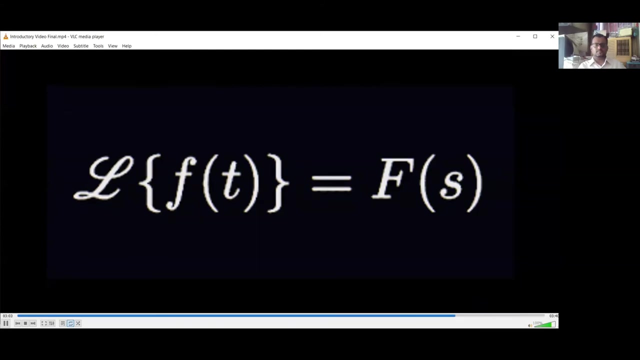 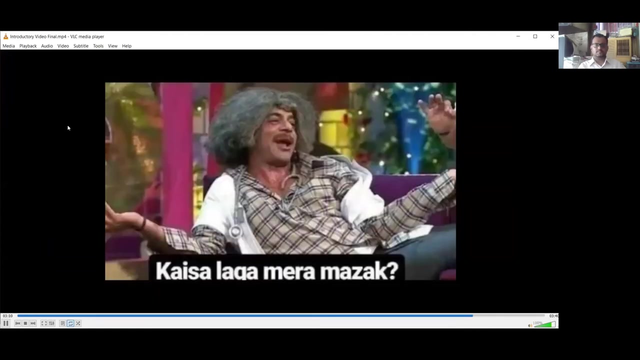 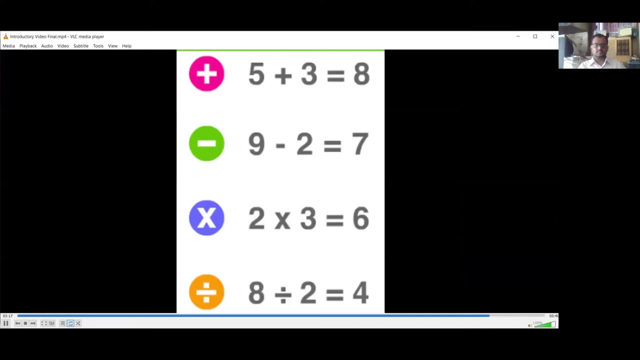 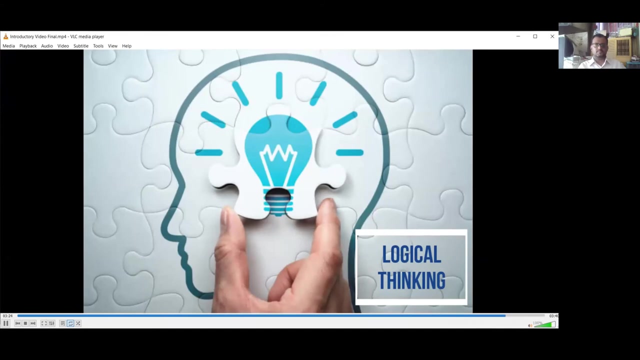 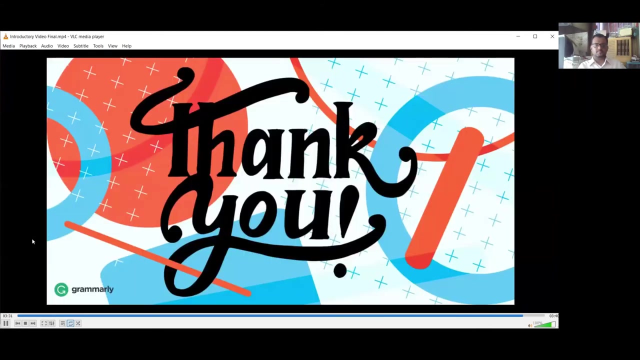 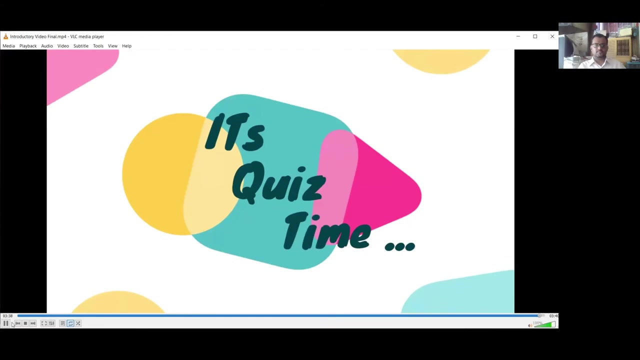 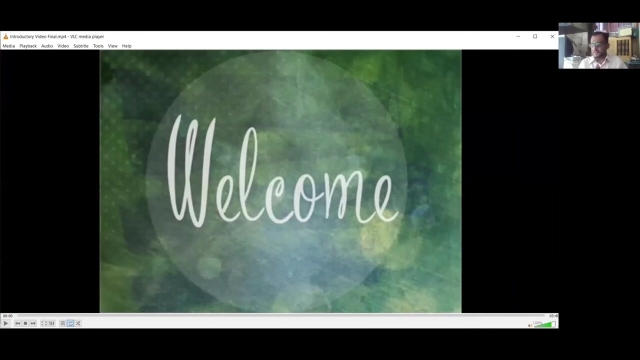